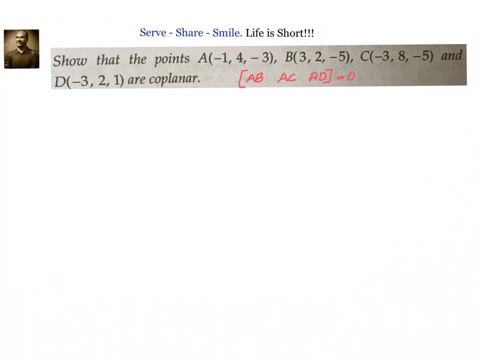 the position vectors of A, B, C, D. Let us write down position vectors. I will write down PVs first for A, then B here, then C here and then D here. A position vector is minus i plus 4j, minus 3k. 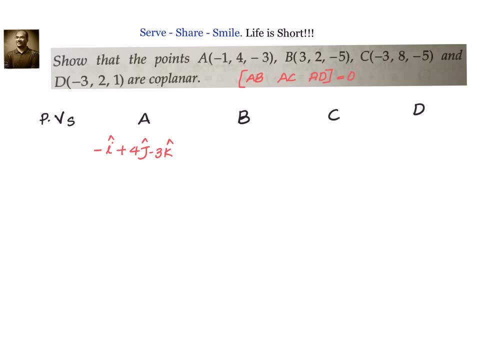 We have caps, unit vectors. they are all For B, what it is 3i plus 2j minus 5k. that is B. Then for C minus 3i plus 8j minus 5k. 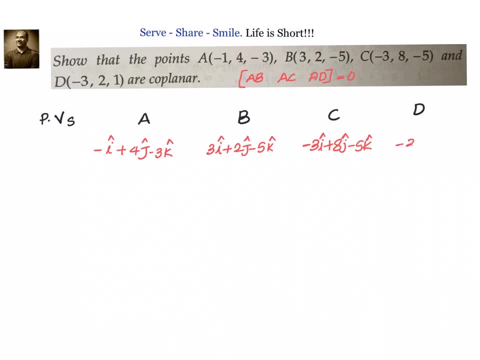 Then D is minus 3i plus 2j, minus 5k, 2j plus k. Now these are position vectors of A, B, C, D. What we need is box of A, B, A, C, A, D. 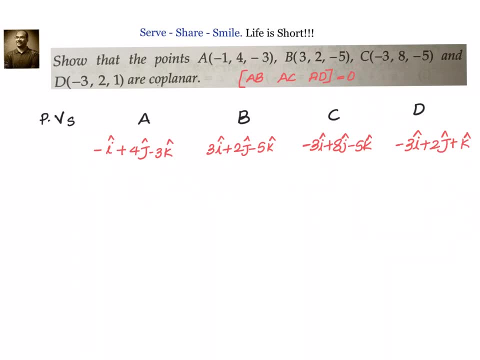 equal to 0.. That is what we need to prove. First, let us find out what is A B vector. A B vector is equal to O B minus O A. That is nothing but equal to 3i. A B vector is equal to O B minus O A. That is nothing but equal to 2j plus 2j minus 5k minus minus i plus 4j minus 3k cap. 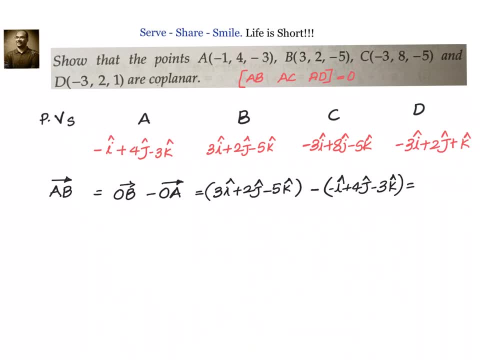 Simplify this: 3i minus of minus i, that is 4i. 2j minus 4j, that is minus 2j. Then minus 5k plus 3k, that is minus 2k. So this is A B. Then we will find out what is A C. 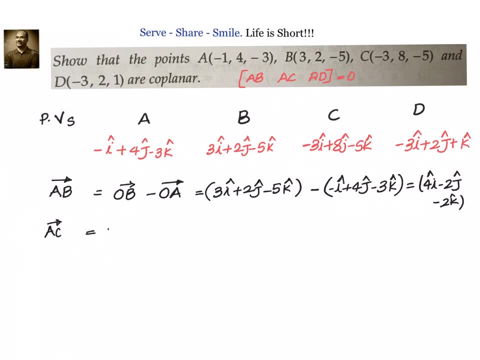 A C vector is equal to O C minus O A. What is O C? That is minus 3i cap plus 8j minus 5k minus O A. That is minus i plus 4j minus 3k. 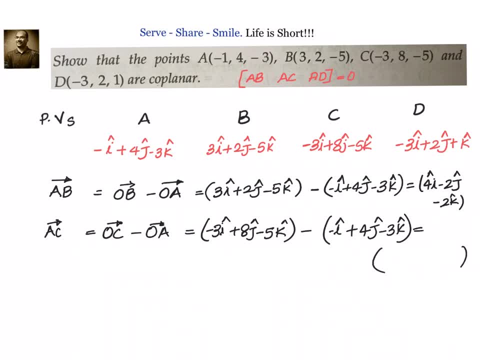 And that simplifies to minus 3i plus i, that is minus 2i. Then plus 8j minus 4j, that is plus 4j. Minus 3i, plus 4j, that is minus 2i. 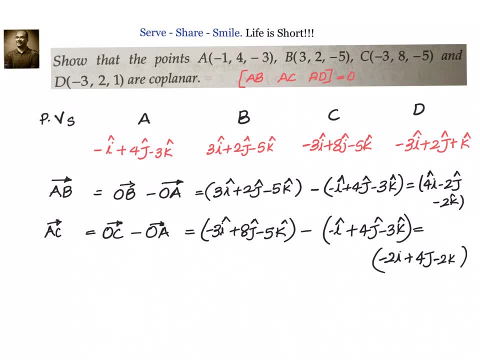 Minus 5k plus 3k, that is minus 2k. Now that is A C. Let us calculate now what is A D A, D is O D minus O A. Now what is D? We have minus 3i plus 2j plus k, minus i plus 4j. 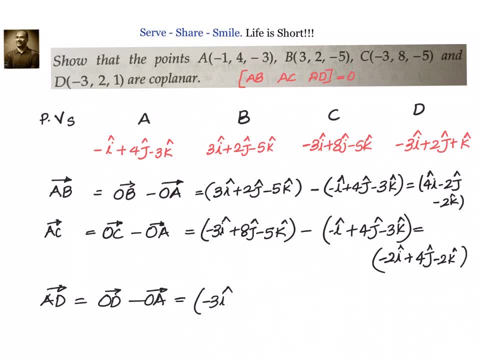 Now what is D? We have minus 3i plus 2j plus k, minus i, plus 4j Minus 3i plus 3i plus 2j plus k minus i plus 4j Minus 3k, minus 3k. that is equal to minus 3i plus i, which is equal to minus 2i. 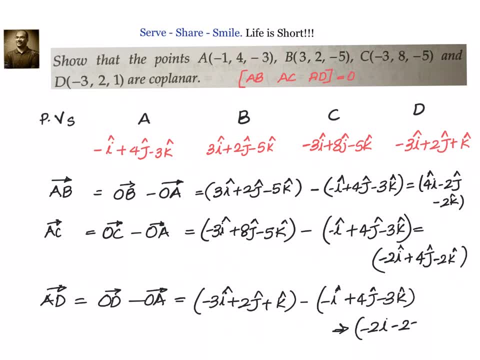 Then 2j minus 4j, which is minus 2j. Then k minus of minus 3k, that is plus 4k. Now we have A, B, A, C, A, D. Now we have to just prove that box of this is equal to 0.. 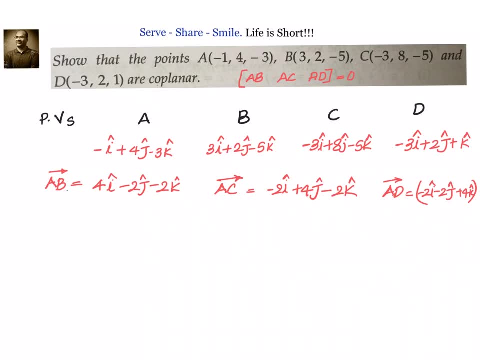 Box of A, B, A, C, A, D equal to 0, we know is nothing, but the debt is equal to 0. So let us write down. We have to prove that debt is equal to 0.. So box of A, B, A, C, A, D is equal to debt of 4 minus 2, minus 2, minus 2, 4, minus 2.. 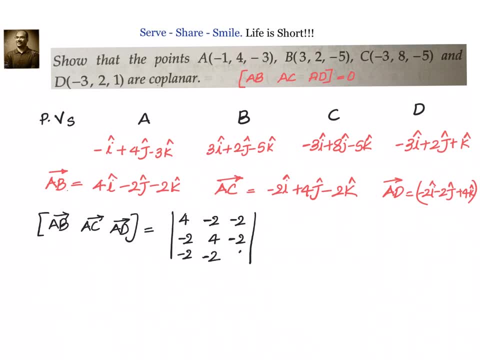 Minus 2,, then minus 2, and 4.. Now this we have to prove equal to 0.. Now let us simplify this. From the first row, I will take 1, 2 out. From the second row, I will take minus 2.. 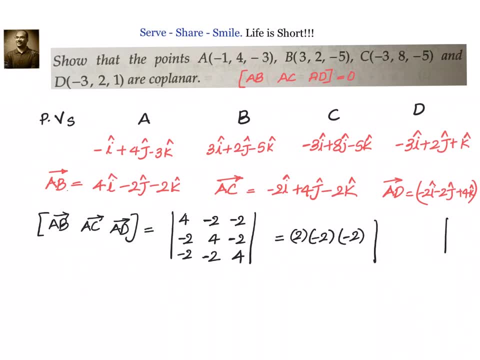 From the third row, I will take minus 2.. So what is left out? First row will have 2, minus 1, minus 1.. From the second row, we will have 1, minus 2, 1.. 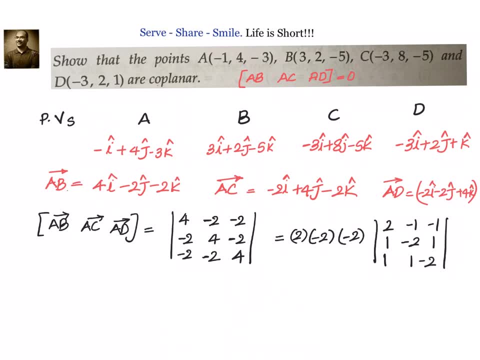 And from the third row we will have 1, 1.. Minus 2.. Now what I will do is I will write down: R1, R3 is assigned, R3 plus R2 plus R1, whole thing divided by 2.. 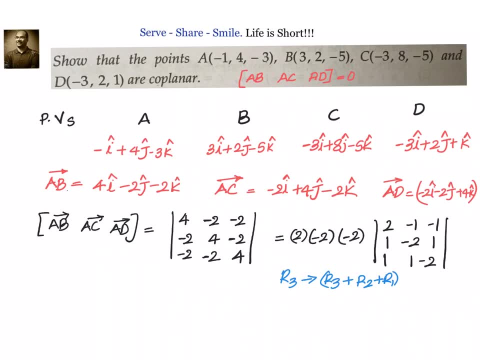 Or we can just keep it. R3 is assigned R3 plus R2 plus R1.. Now see what happens. In the next step we will have 8.. R1 will be 2, minus 1, minus 1.. R2 is 1, minus 2, 1.. 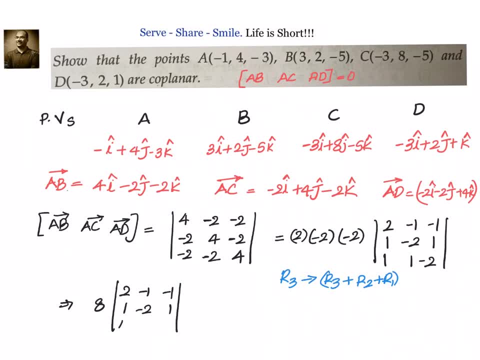 When we do R3 is assigned R1 plus R2 plus R3, we will have 4. Then we will have minus 2. And then we will have minus 2.. Now you can see very clearly R1 and R3 are related. 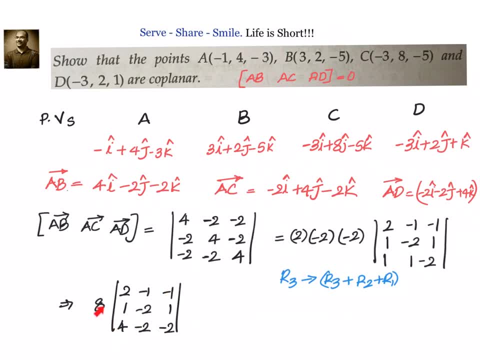 R3 is 2 times of R1. So let us take 2 out from the last row, Then we have 2 identical rows. We can write down 16 into 2, minus 1,, 2, minus 1, minus 1.. 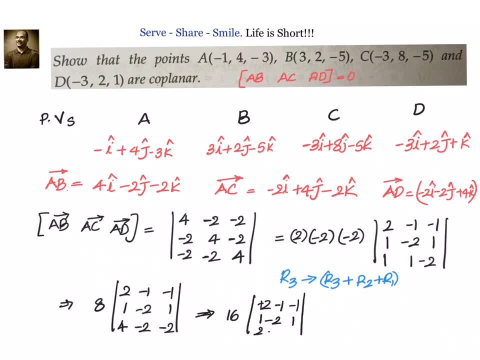 Then 1, minus 2, 1.. And also 2, minus 1, minus 1.. Now we can say that R1 and R3 are identical. That means that equals to 0.. That means that is equal to 0.. 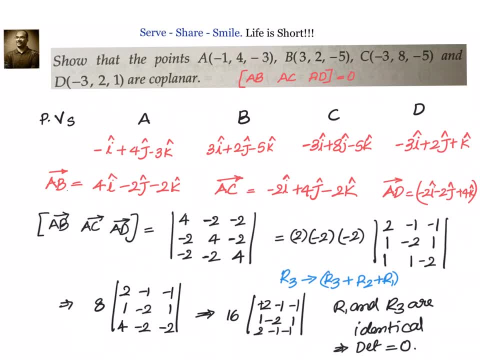 Now, once we get that, equals to 0.. What we have proven now is that A, B, A, C, A, D are coplanar. If A, B, A, C, A, D are coplanar, automatically points A, B, C, D are coplanar.